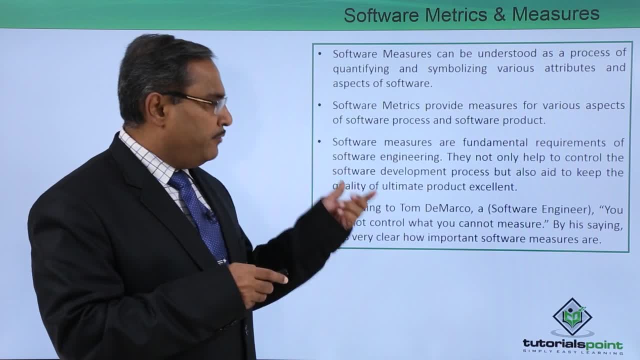 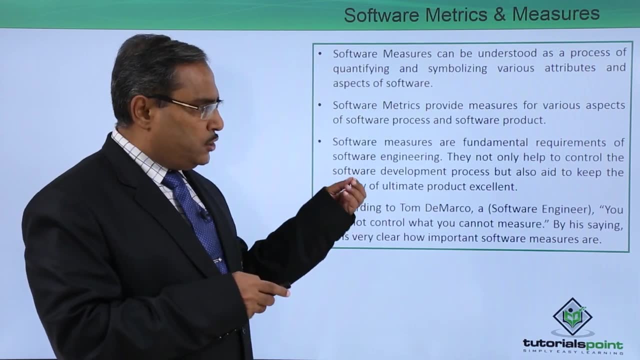 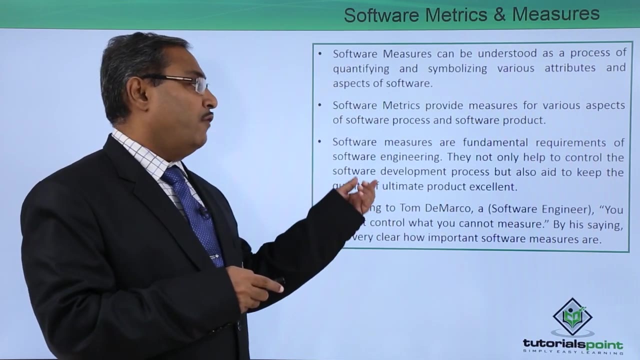 software product. So software measures are fundamental requirements of software engineering. Ultimately, software is an engineering product, So they not only help to control the software development process but also aid to keep the quality of ultimate product excellent. So if you 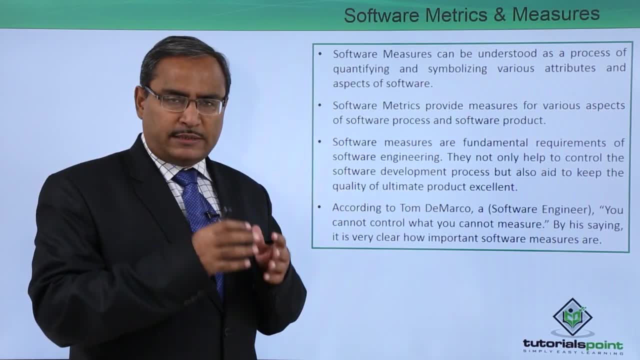 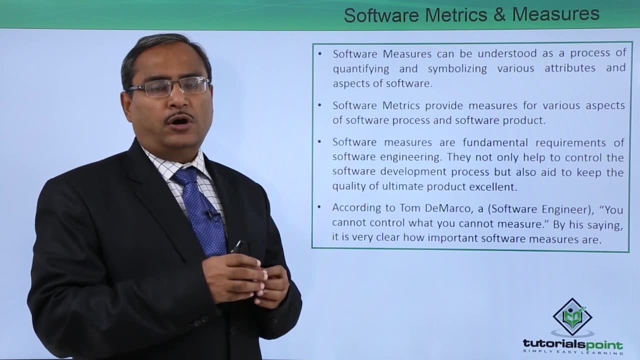 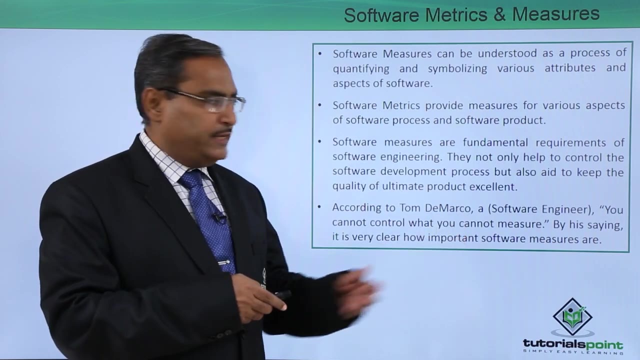 can go on doing some measurements, having some metrics in different aspects of the software, So that will also ensure that how for good quality of software we are going to develop. So according to is one of the very famous software engineer. he has made one statement: that you cannot control what you. 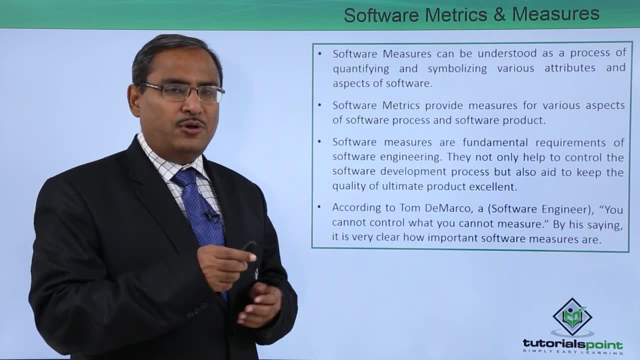 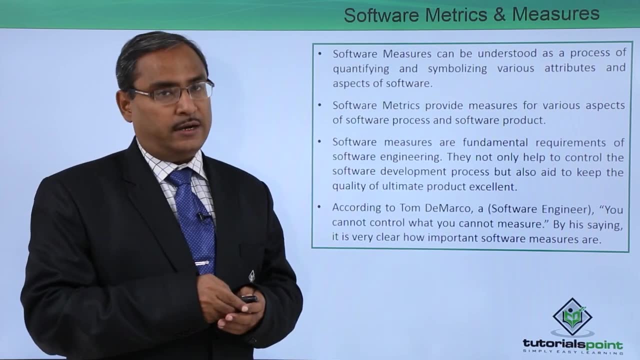 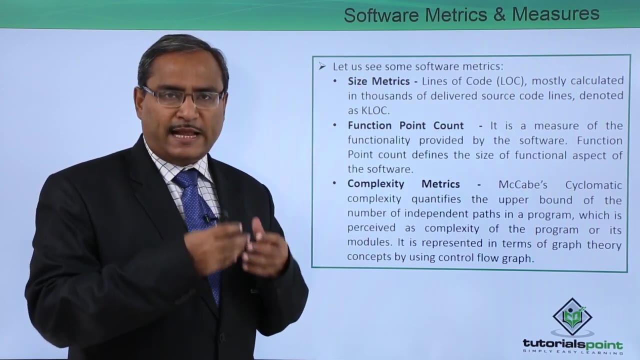 cannot measure. So that is very interesting. You cannot control what you cannot measure. So by saying it is very clear that how important the software measures are. So now let us go for some software metrics: How to do this software, What are the different aspects of software metrics? So size. 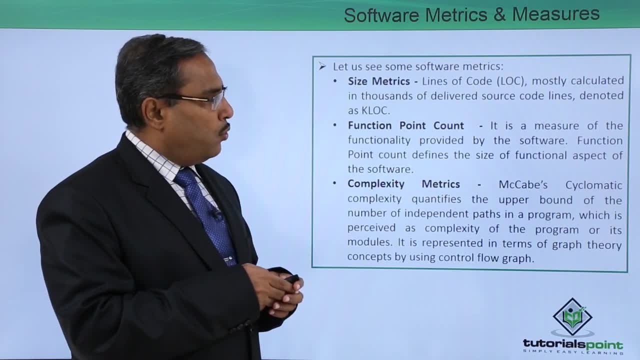 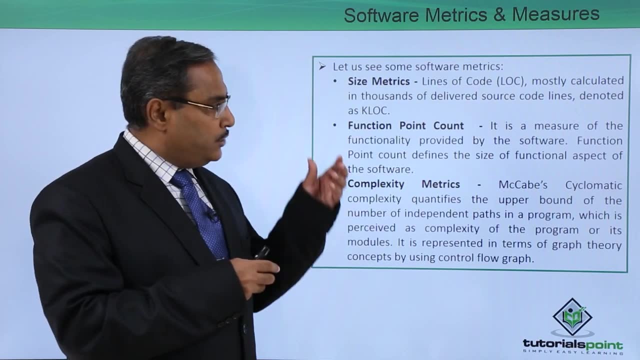 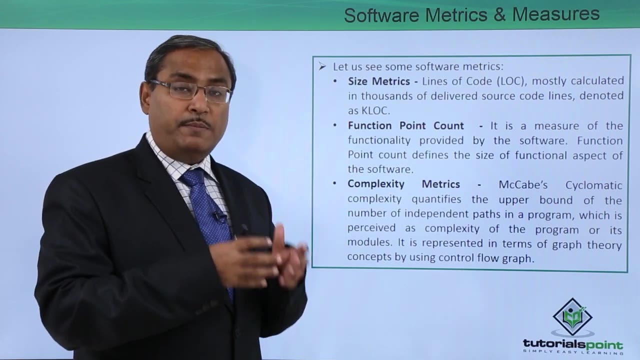 metrics. So, first one, we are considering The lines of code, that is the LOC, and mostly calculated in thousands of delivered source code lines. In short, it will be denoted as KLOC. So, depending upon the value of this KLOC, the software metrics. 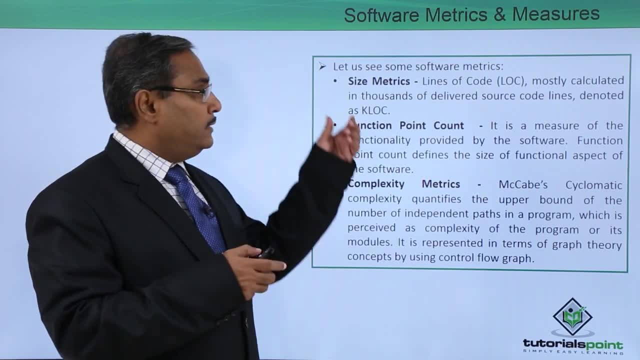 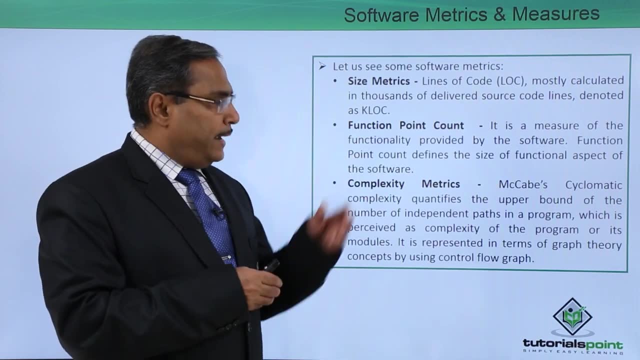 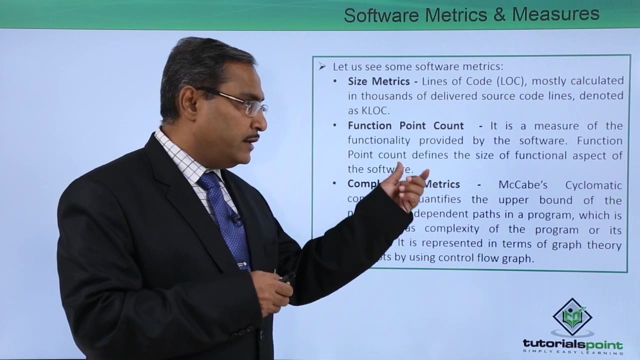 can be done, The measurements can be done and this size metrics is one of the metrics of that measurement: Function point count. It is a measure of the functionality provided by the software. So function point count defines the size of functional aspect of the software. We know that each and every 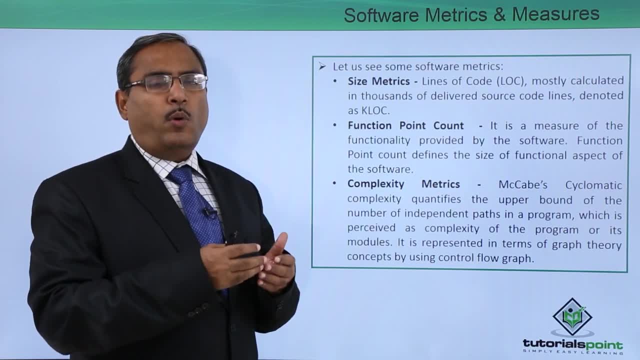 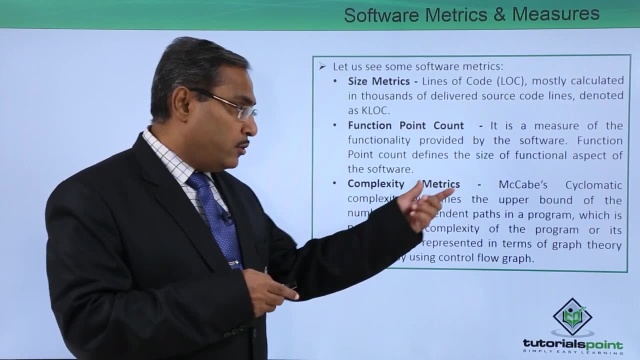 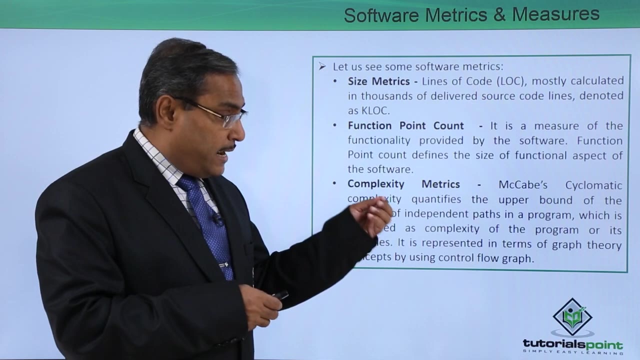 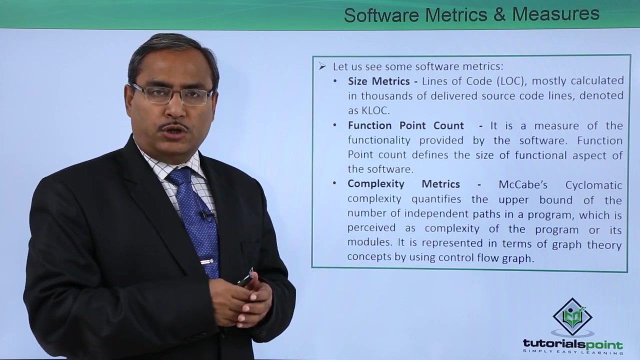 function point is actually implementing one of the functional requirements of the software: Complexity metrics. So Maccab's cyclometric complexity quantifies the upper bound of the number of independent paths in a program which is perceived as complexity of the program or its modules. So how many number of independent paths are flowing through a software? So that will be. 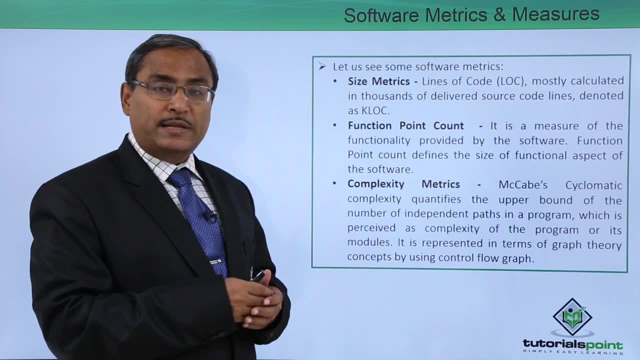 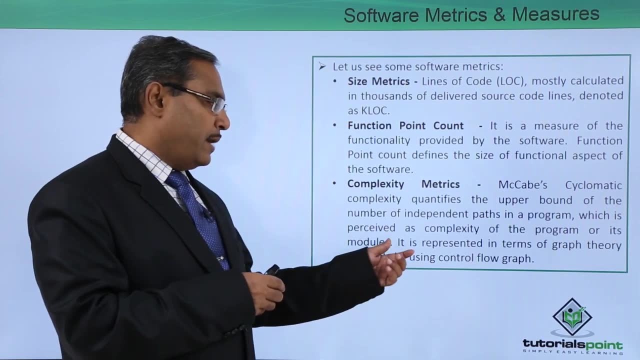 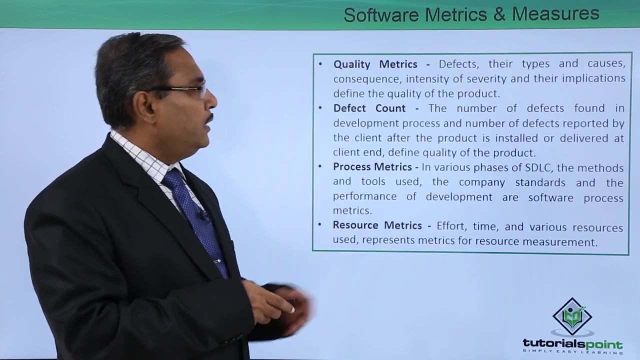 also another metric and this metric is known as complexity metrics, and that is a psychometric complexity. So it is represented in terms of graph theory concepts by using control flow graph. So we are having a separate video on this respective aspect. So quality metrics, So defects, their types and causes. 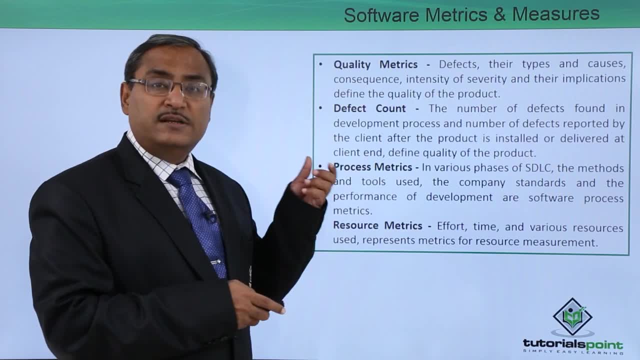 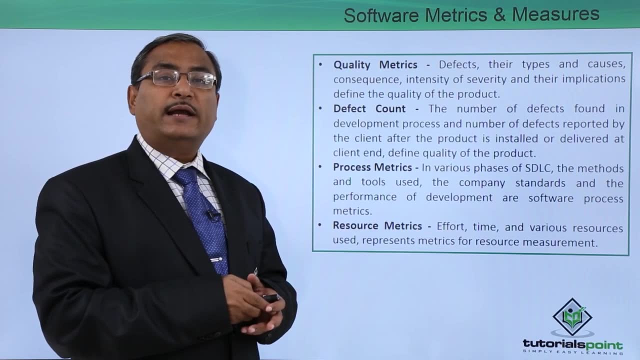 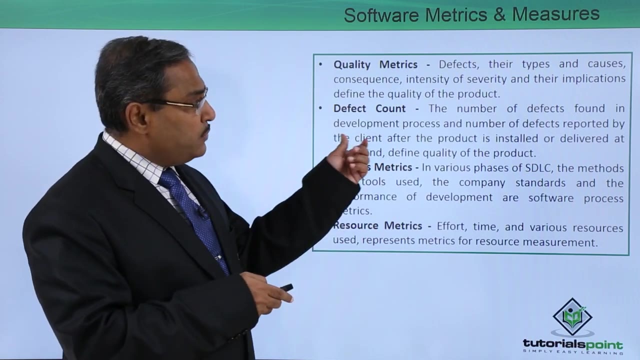 Consequence. intensity of severity and their implications define the quality of the software. So in our software we are doing different kinds of risk managements, So each and every risk should be done some intensity values. So that is why we are having the intensity of severity and that implication defines the quality of the 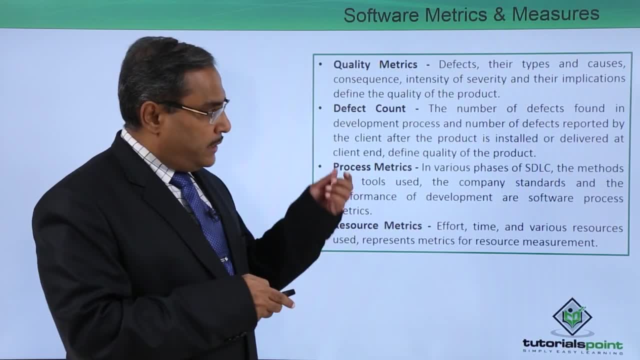 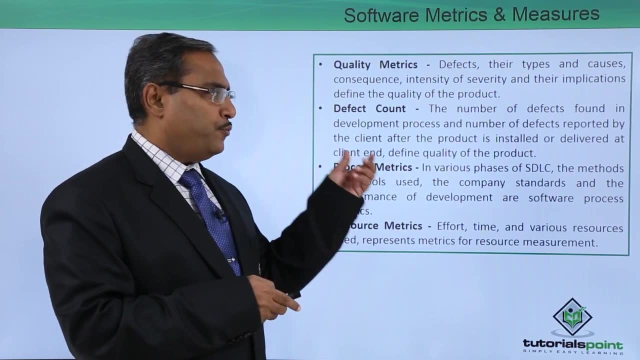 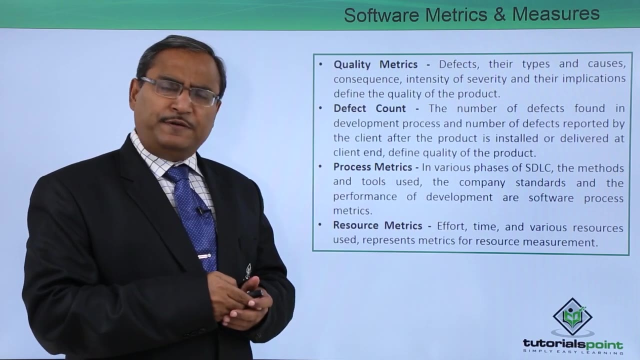 software. Next one is the defect count. The number of defects found in the development process are. the process and number of defects reported by the client after the product is installed or delivered at the client end define the quality of the product. So defect count is a very important. 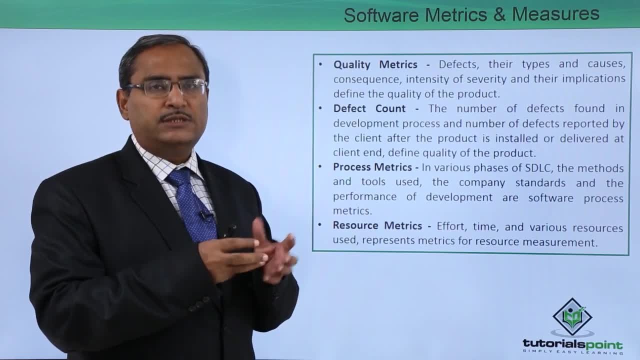 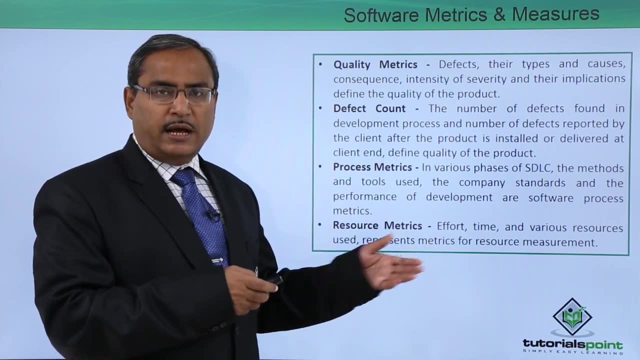 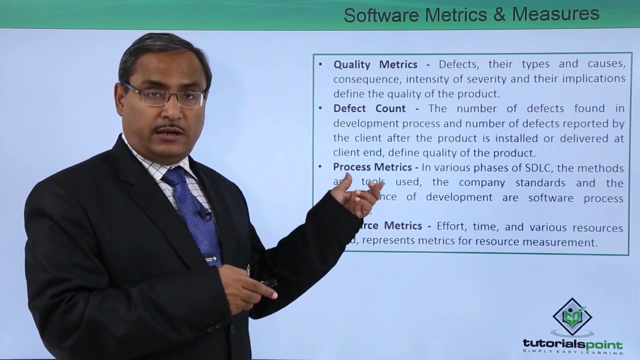 and very obvious measures and metrics for this software quality. So how many defects has been detected after getting it installed at the customer side, and how many, against how many defects the customer has put the feedback? So that might be also a good metric to decide the 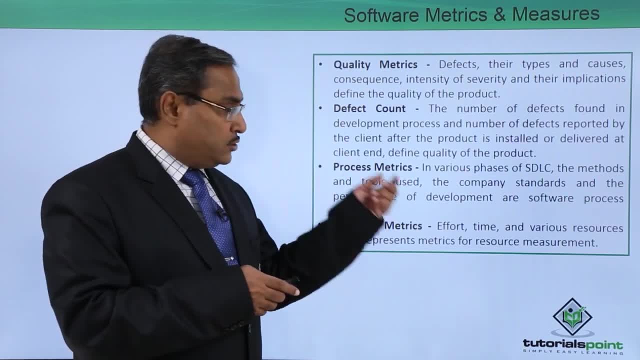 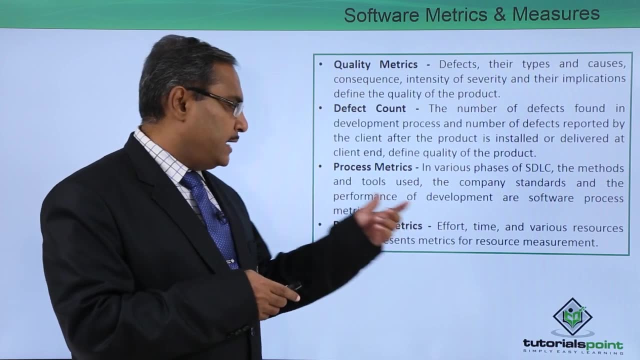 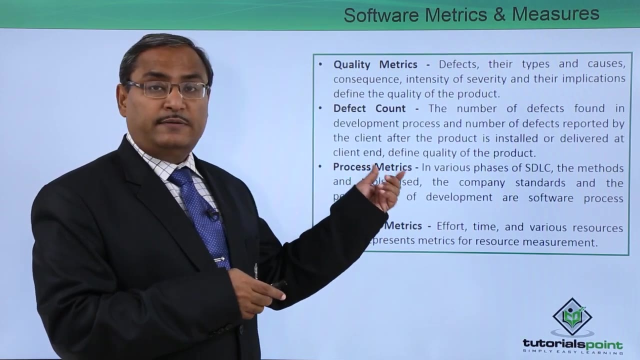 quality of the product Process metrics. So, in various phases of SDLC, the methods and tools used, the company standards and the performance of development are the software process metrics. So what are the different in case of different SDLC? the methods and the tools, whatever we have? 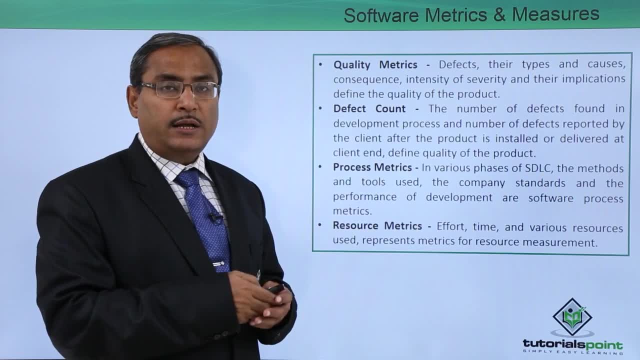 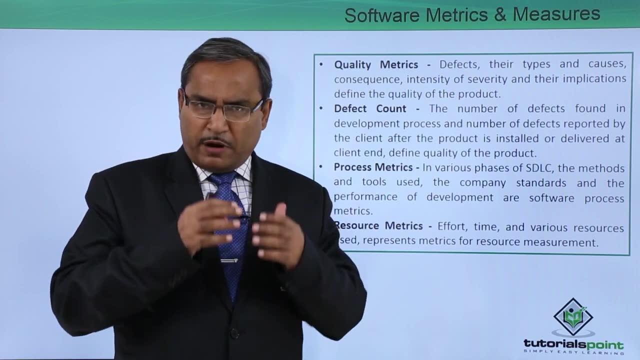 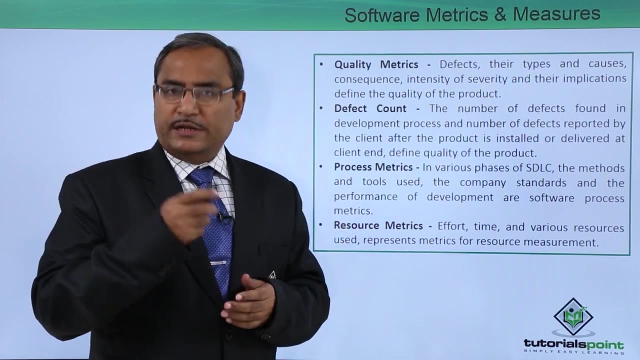 used, So that might be also another metrics known as the process metrics. Next one is our resource metric. there is a effort, time and different resources deployed on that very particular software will be a good measure for our resource metrics. So now in our earlier video also. 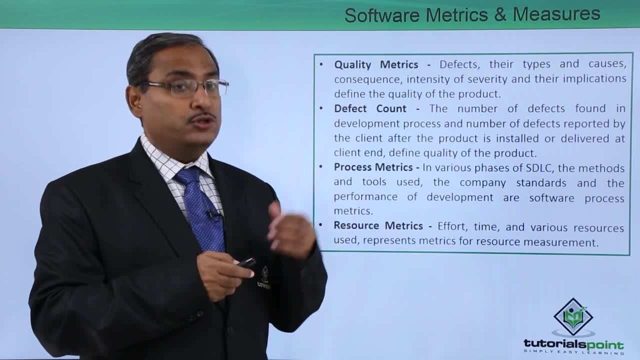 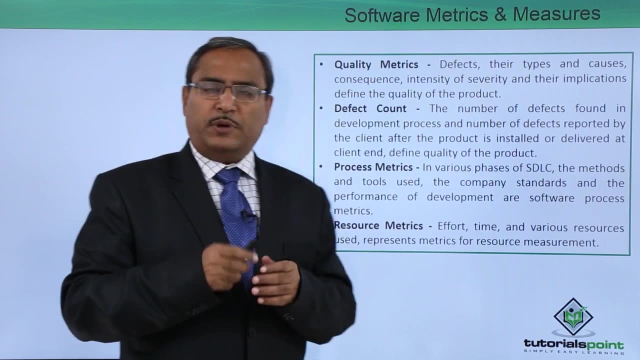 we have discussed a lot on this resource management and all. you can also have a look on those videos for the better understanding. So that is why, in this particular video, we have discussed the software metrics and the respective measures. Thanks for watching this video.